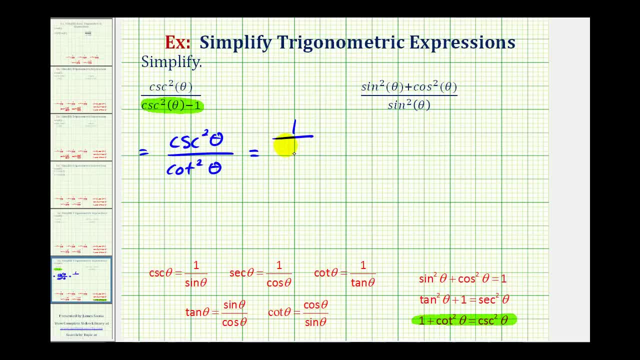 cosecant squared theta would be one over sine squared theta. And since cotangent theta is equal to cosine theta over sine theta, cotangent squared theta will be cosine squared theta divided by sine squared theta. Now this fraction bar here represents division, so we can write this as a division problem. 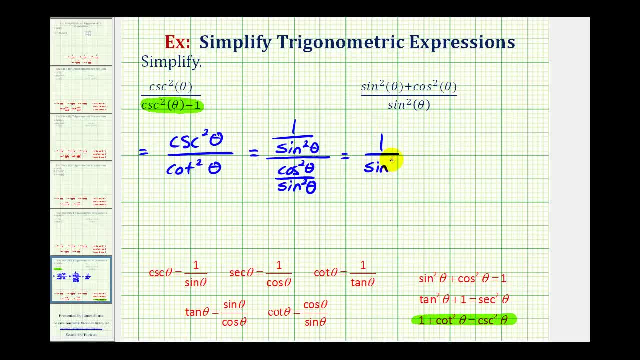 So we'd have one over sine squared theta, divided by sine squared theta, Divided by cosine squared theta over sine squared theta. And now we can write this division problem as a multiplication problem if we multiply by the reciprocal of this fraction here. So let's go ahead and do that. 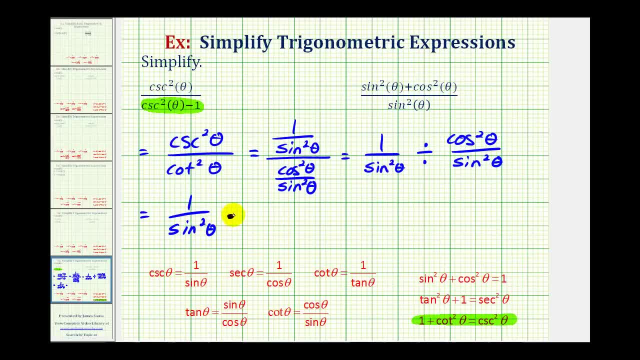 So we have one over sine squared theta times the reciprocal of this fraction. So we'll have sine squared theta over cosine squared theta and in this form notice how sine squared theta over sine squared theta simplifies to one. So this simplifies to one divided by cosine squared theta. 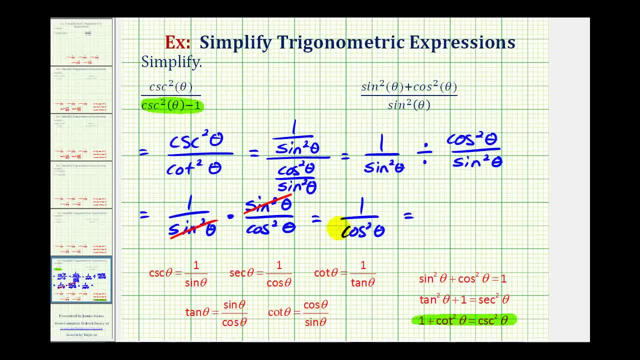 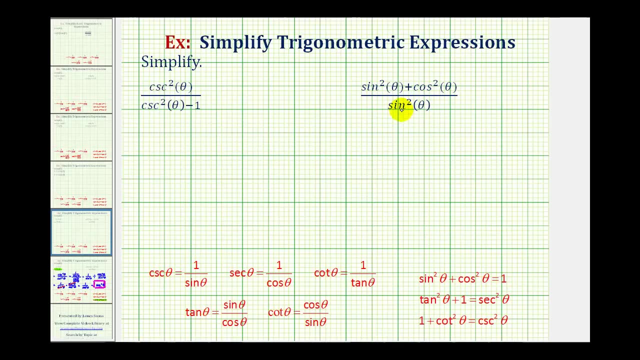 But since one over cosine theta is equal to secant theta, this simplifies nicely to secant squared theta. Let's take a look at our second expression on the next slide. Because our denominator does not contain a sum or difference, we could break this up into two separate fractions. 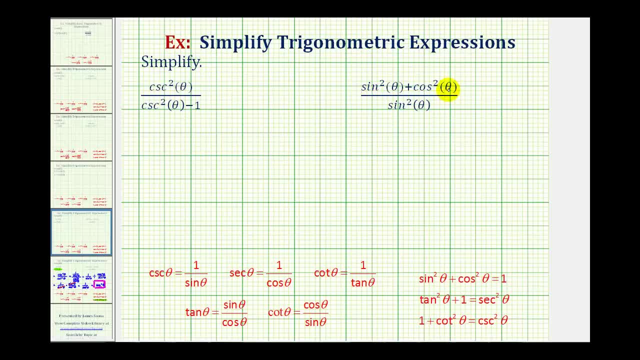 and simplify this. But again, because we have trig functions that are squared, we should look at the Pythagorean identities. first Notice: here we have sine squared theta plus cosine squared theta equals one. This is a perfect match for our numerator. We can substitute one for sine squared theta. 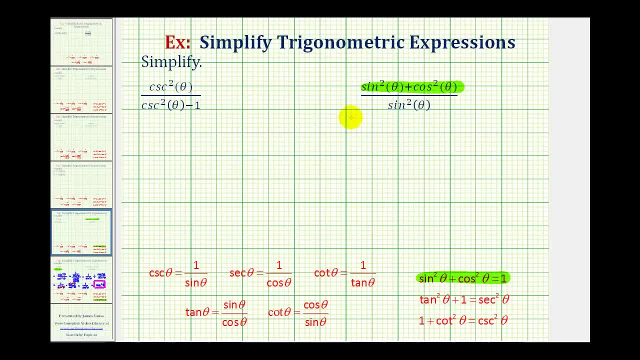 plus cosine squared theta. So this simplifies very nicely to just one over sine squared, which is one over sine squared theta, And since one over sine theta is equal to cosecant theta, this simplifies to cosecant squared theta And that's going to do it for these two examples. I hope they were helpful.